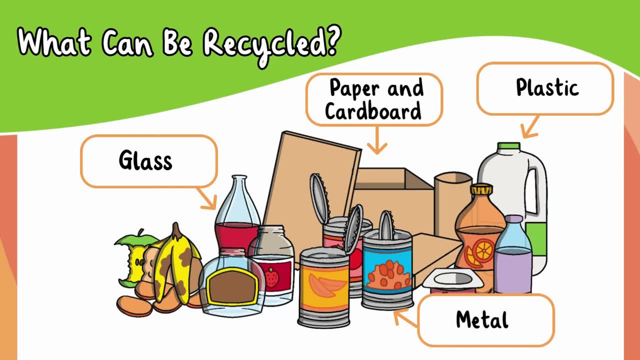 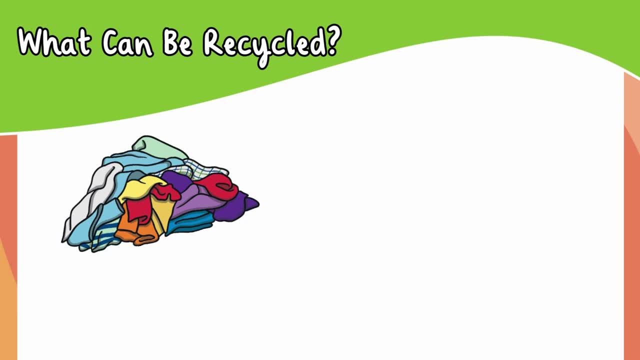 off a special gas that can be used to make electricity. Clothes can be recycled by donating them to charities so that other people can wear them. They could also be used to stuff furniture. Used cooking oil can be turned into something called biodiesel, which can be used to fuel trucks. 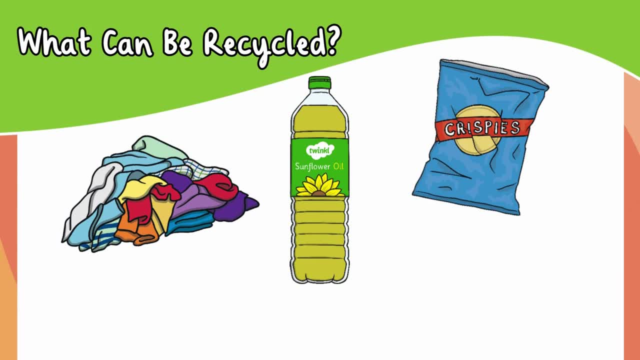 Things like chip bags and food patches are a bit more tricky to recycle, but some special companies can do it. Leaves or grass cuttings can be turned into compost, which helps soil. We can put our recycling into the recycling bin at home or school. 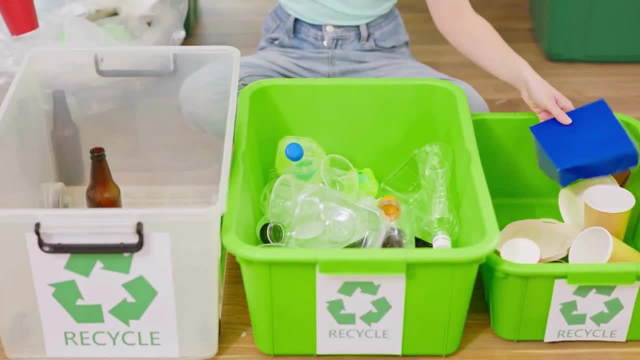 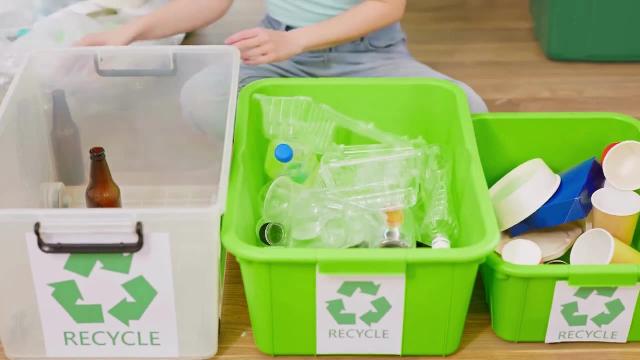 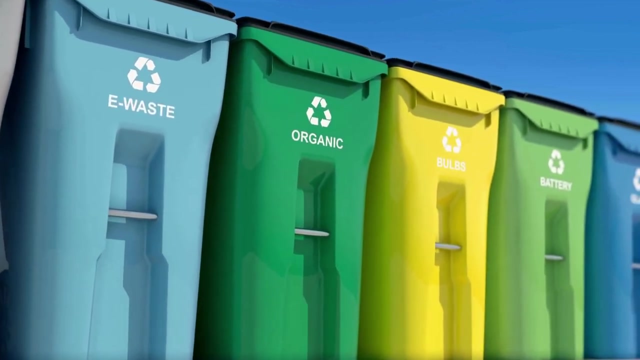 In certain places you may need to separate the cardboard and paper, metal, glass and plastics, but sometimes they can all go in one big bin or bag. Look out for recycling stations when you're out and about in your local area. Have you ever wondered what happens to your recycling? 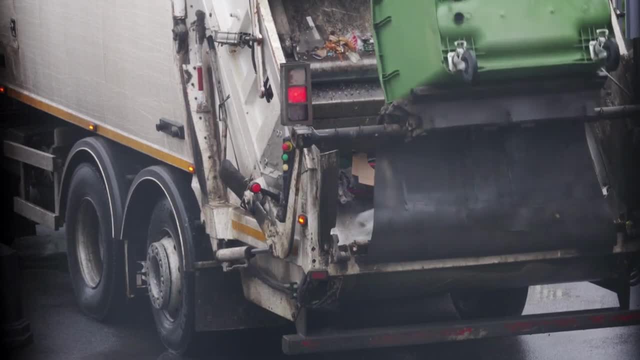 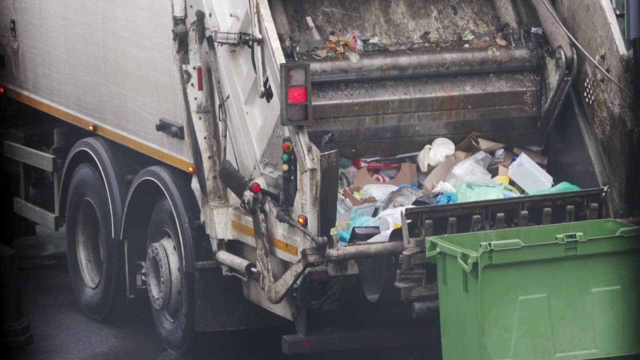 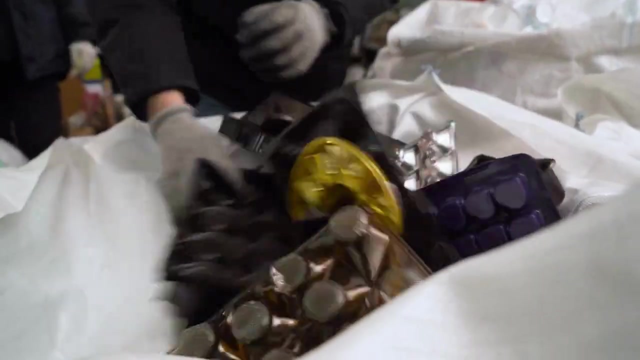 After you've put it in the recycling bin, Let's find out. A recycling truck comes to collect the trash from outside your home and then takes it to a place called a recycling facility. At the recycling facility, everything is sorted and put into big bundles before 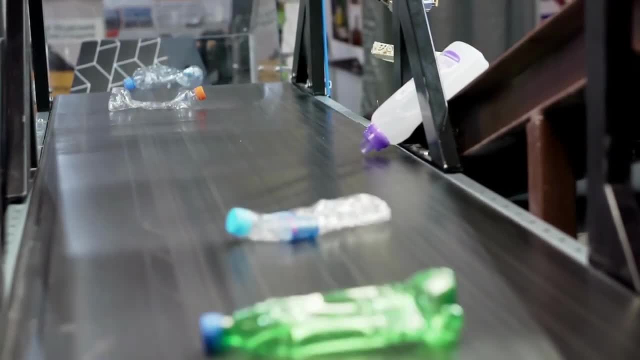 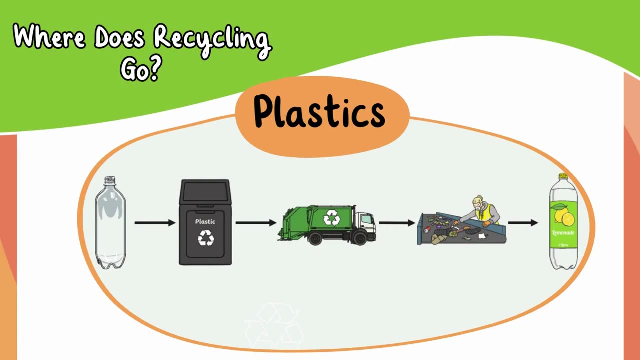 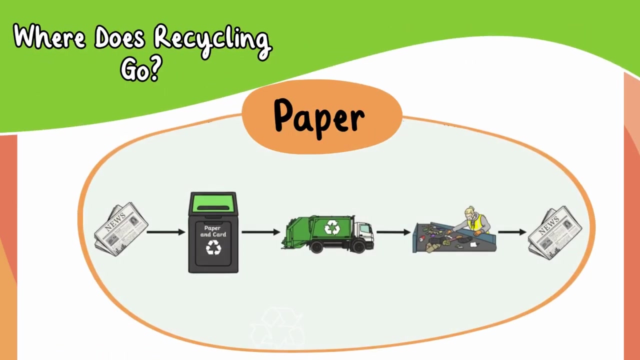 being taken to factories to be turned into something new. Plastics can be turned into new bags, bottles and even t-shirts. Plastics are shredded into little strips before also being melted and made into new things. Paper is washed in soapy water. It is then mixed and rolled out before being left to dry. 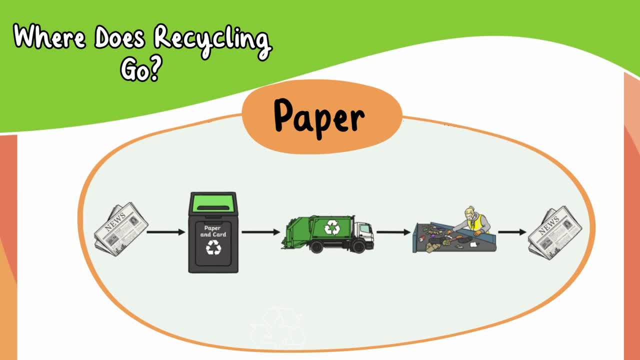 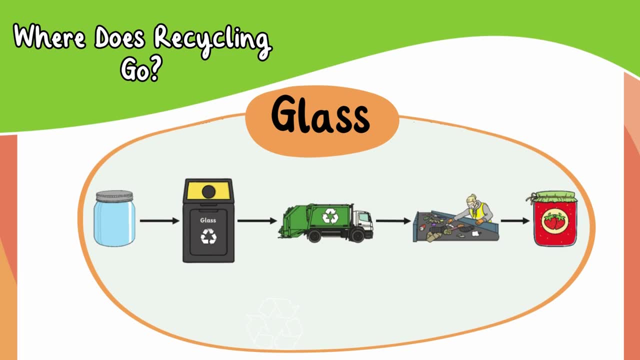 It is then turned into different types of new paper and cardboard, such as newspapers. Machines sort glass into different colors. It is then crushed into tiny balls, heated up and melted into liquid glass. The liquid glass can then be molded into the shape of new bottles or jars before it cools down and becomes hard again. 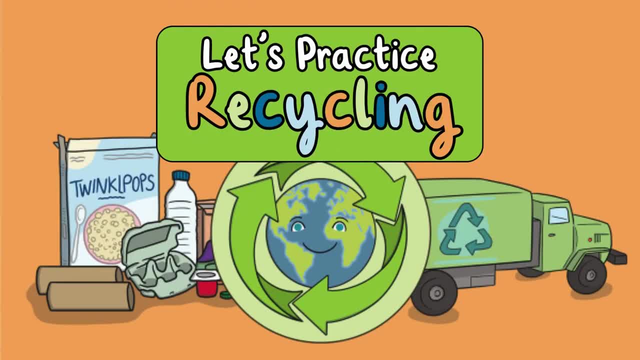 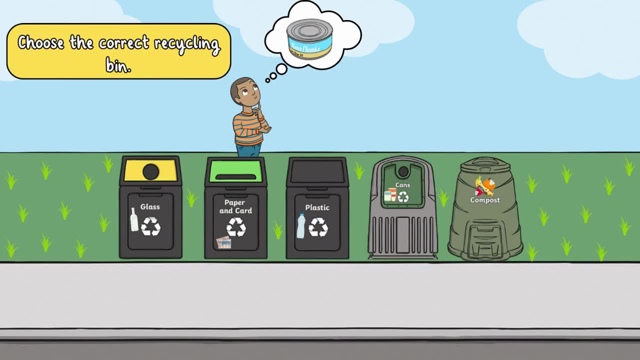 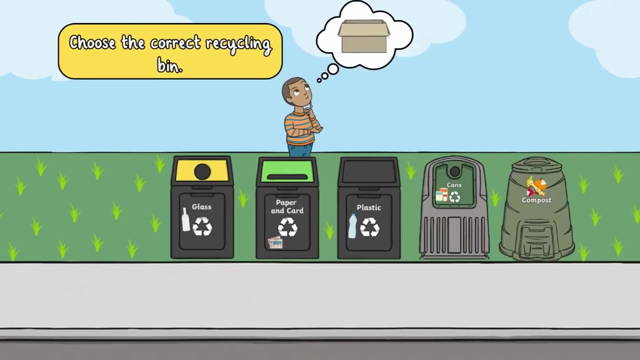 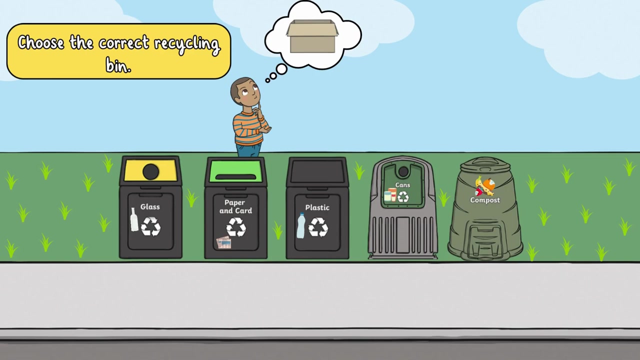 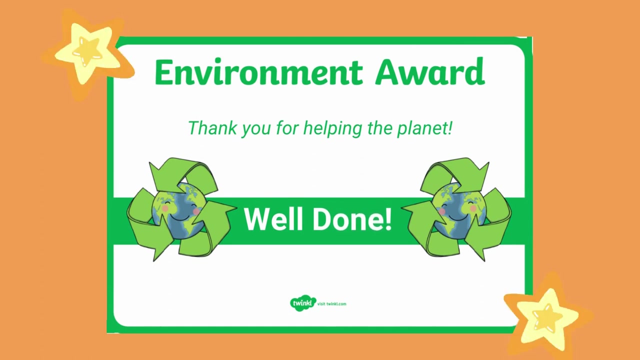 Let's practice recycling. Choose the correct recycling bin Cans. Cans, Paper and card Plastic Cans. Cans Compost Compost Glass, Paper and card. Glass Compost Plastic. Well done and congratulations: You received an Environment Award. Thank you for helping the planet. 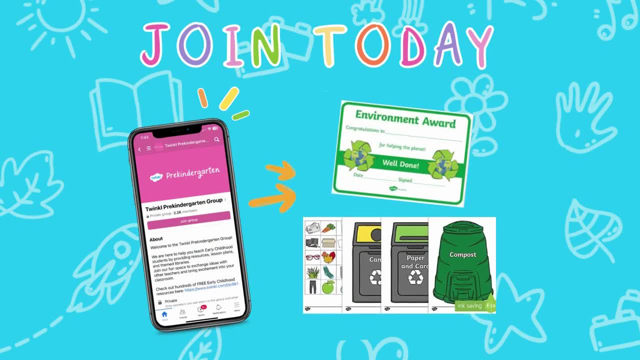 Teachers join the Twinkle Pre-Kindergarten Facebook group to get a free Environment Award printable certificate and a recycling sort activity. For more information, visit wwwtwinklecom.